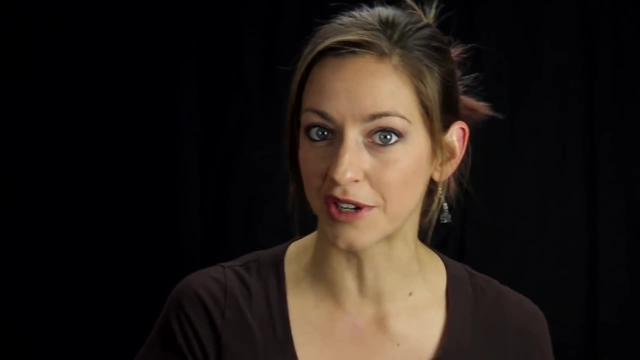 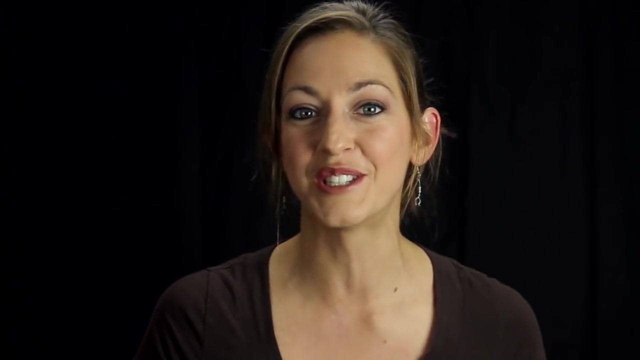 Now most of the focus is on improving encryption, because as computers get smarter and faster, these codes become easier to unscramble. That's why I'm here. That's why we need to turn to cutting-edge physics to improve encryption. 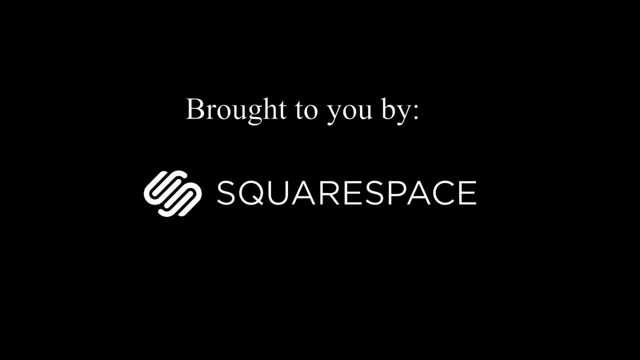 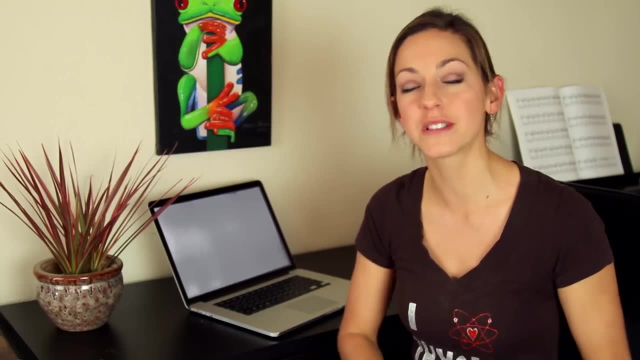 But let's find out how This episode of Physics Girl is supported by Squarespace. Share your passion with the world. Before I go physics on you, let's talk about codes, A super simple type of code, but one that was used by the Spartan army and probably Scooby Doo is simple substitution. 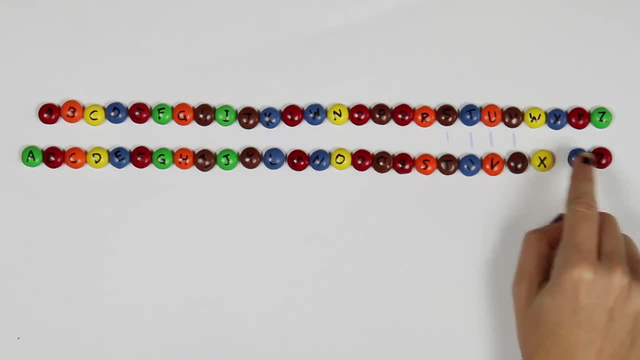 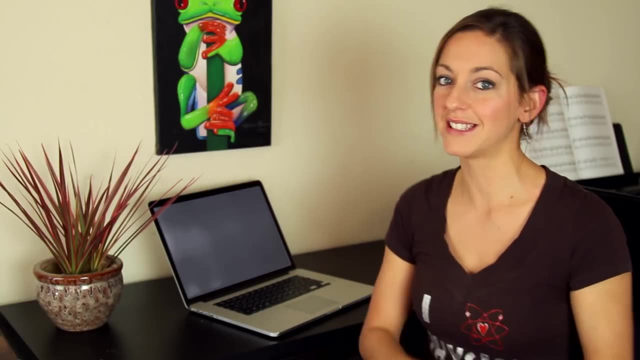 where you just swap out each letter in the alphabet for a different letter. Like so, For example, Diana Rocks would become EJ Boobs Dolts. This code is easy to generate and almost as easy to craft. You could even use extra information, like guessing that the six-letter word with the double O's was my name. 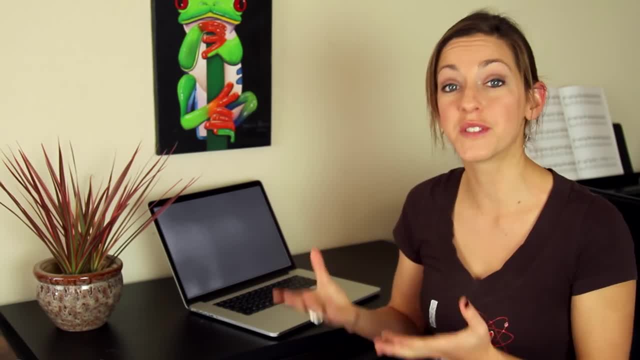 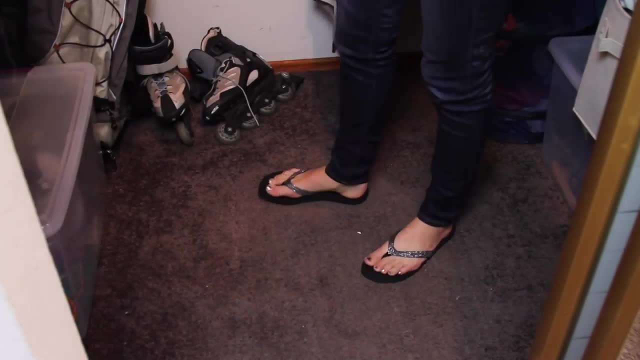 helping you to crack the code faster. So cryptographers turned to math to develop harder codes. They thought a good code should be easy to create but difficult to decode Like a mess In math terms. they sought processes called one-way functions. 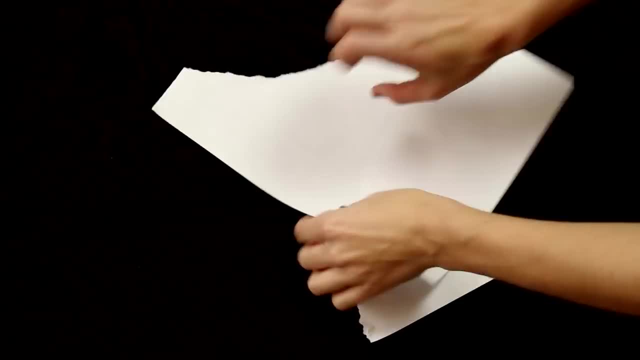 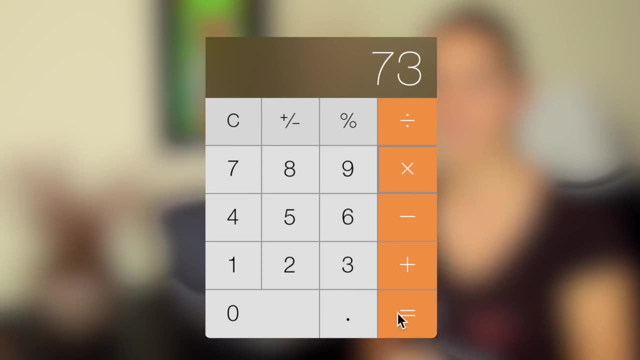 Easy to compute one way but hard in reverse, Like multiplying prime numbers. If I told you to multiply 79 by 73, a few punches on your calculator would give you 50. But if I told you to factor 57 by 67, you'd have to start by saying: does that divide by 2, and then 3, and then 5?? 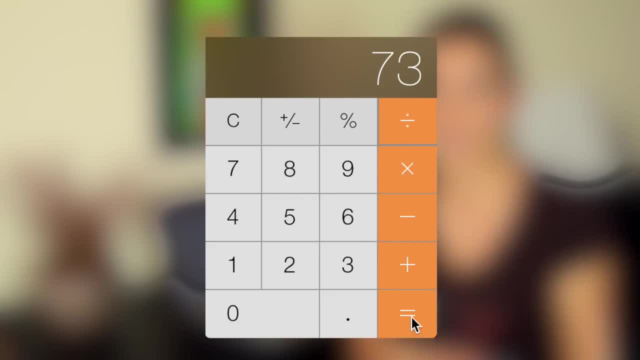 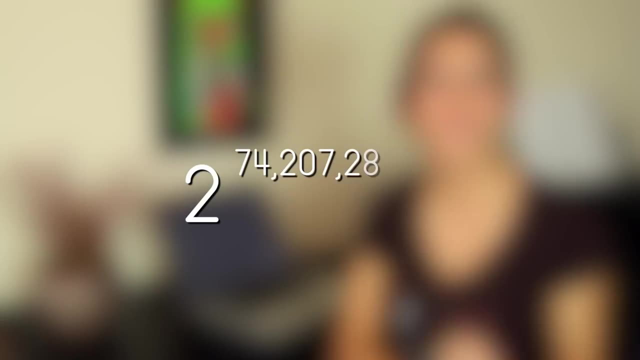 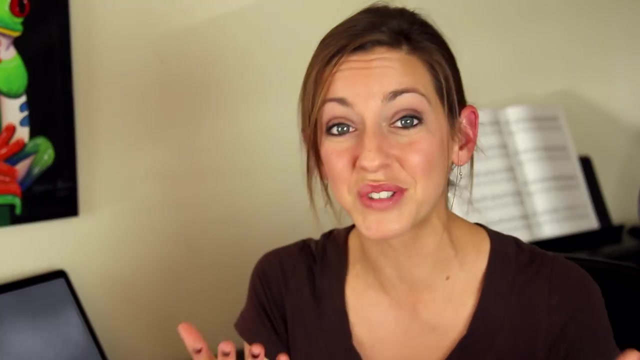 Up through the prime numbers until you finally found 79 times 73. That would take some key punching. The largest prime number known today is 2 to the 74,207,281 minus 1. A number that I couldn't even write on the screen if I wanted, because that's more digits than pixels in my HD video. 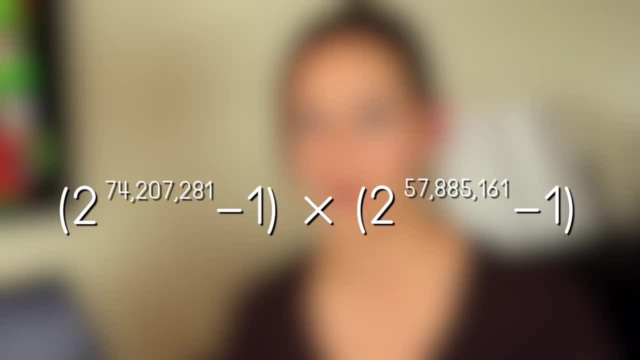 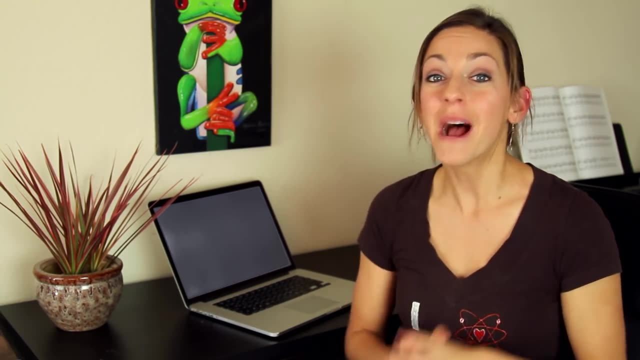 Now imagine multiplying that by the third, That's the second largest known prime number- and giving that to your little cousin to factor on a rainy day. That's just cruel, But it's great for encryption. Imagine I want to send the message Diana Rocks to another secret agent, Sophia. 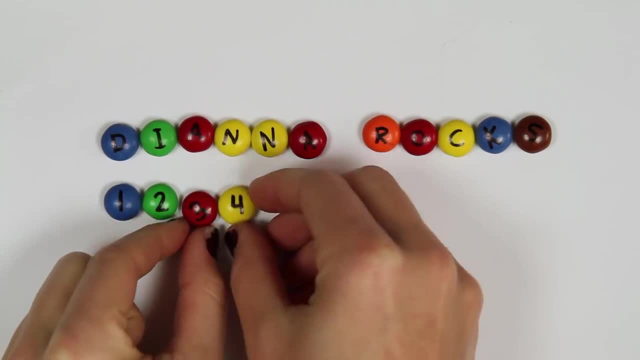 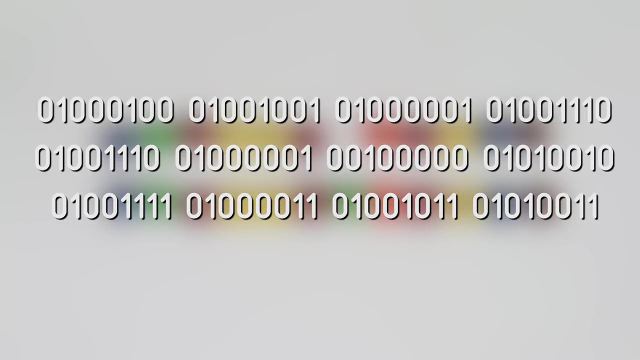 I'm going to use this math. First, I substitute the letters in my message for bits, like we did in our easy Scooby-Doo code. If we were using binary, Diana Rocks would look like this, But we'll just use 1,, 2,, 3,, 4,, 4,, 3,, 5,, 6,, 7,, 8,, 9,, 10.. 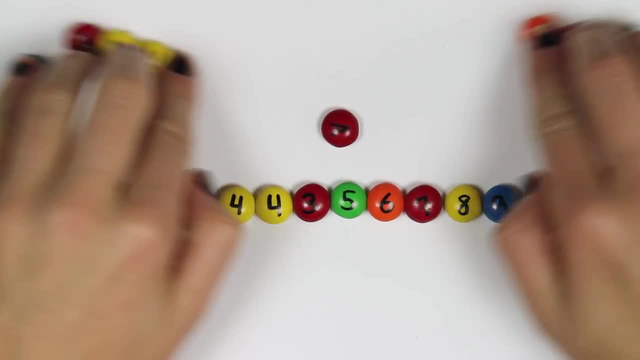 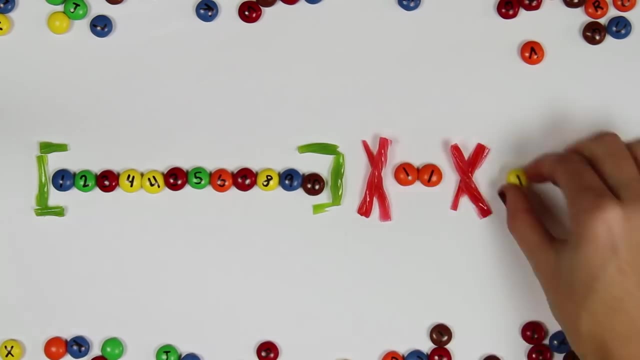 The 5 is for the space. The inversion key from numbers back to letters is publicly known. No surprises yet. But then I multiply each of the numbers by two prime numbers, say 11 and 13,, for a total multiplication factor of 143.. 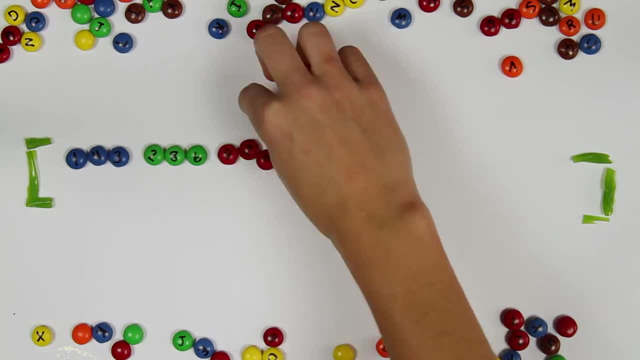 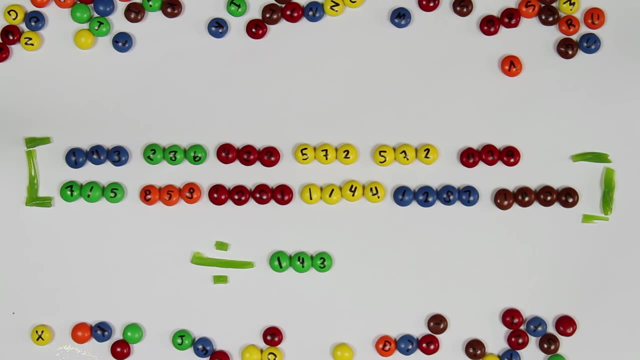 Diana Rocks becomes 143,, 286,, 429, and so forth. I've told Sophia ahead of time that the key is to divide by 143, and she can decode the message. Now, say, someone intercepts the encrypted message. They have to figure out what to divide by to decode the message. 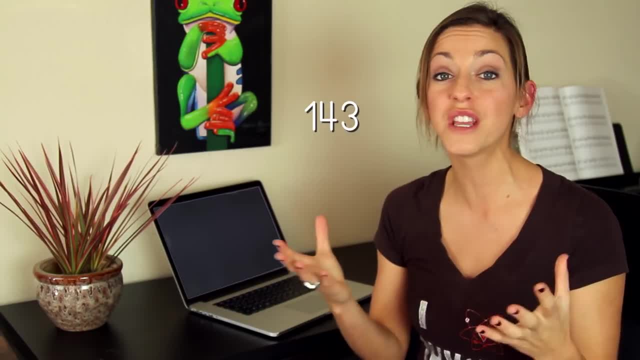 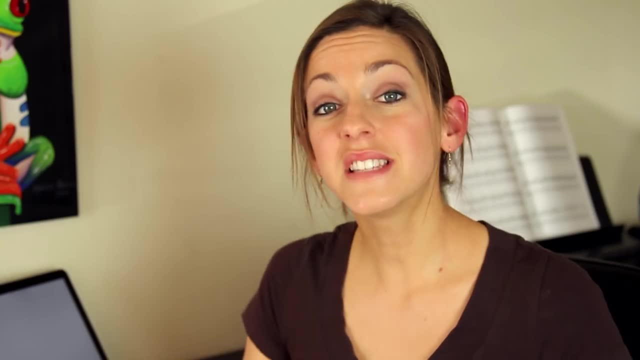 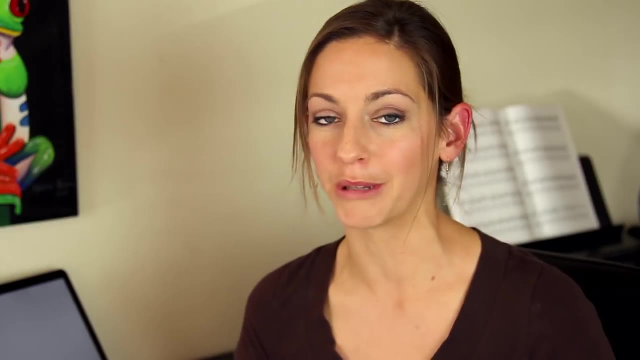 This example wouldn't be so difficult. But what if we used prime numbers that are thousands of digits long? An eavesdropper might be crunching numbers for longer than they are alive. This is the idea behind using prime numbers for encryption, though real-life techniques like the RSA algorithm are a bit more complicated. 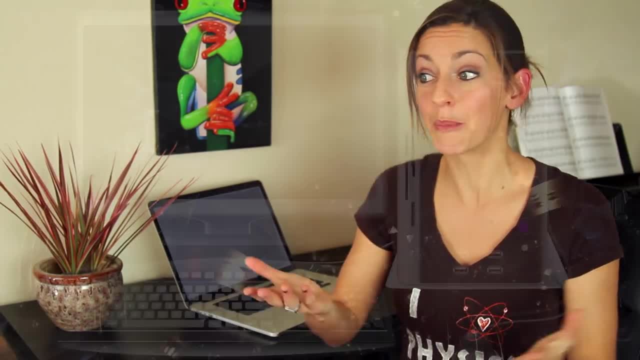 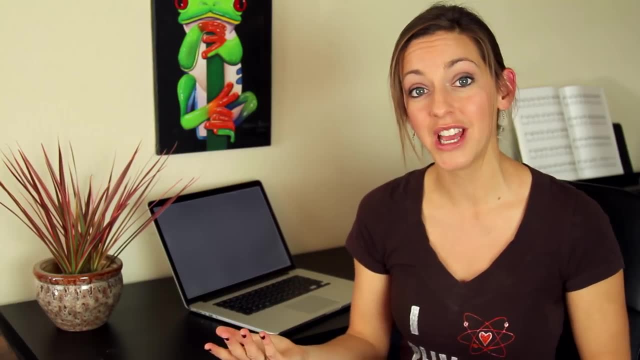 Now the limitation with using prime numbers is that we keep building smarter and faster computers that factor out ever more quickly. Experts warn that with new technologies like quantum computing, codes that currently take hundreds of years to crack could be solved within minutes, And this is where the physics comes in. 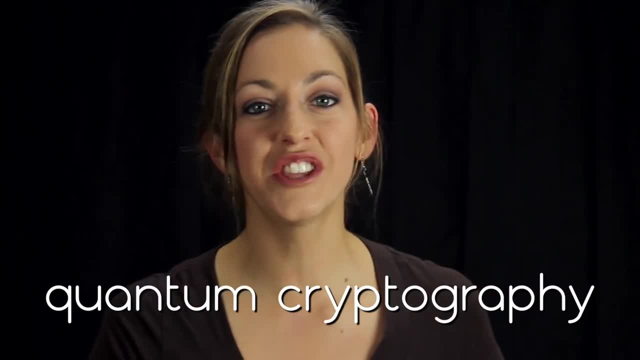 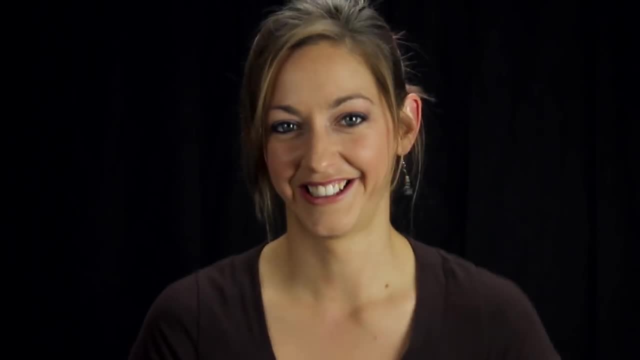 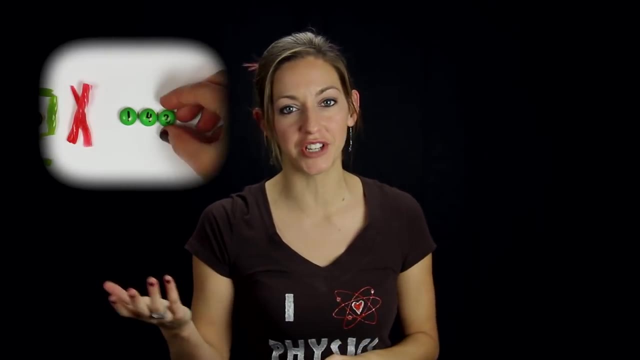 Enter quantum cryptography, a technology that hides information in photons or the particles of light. Here's how it works. Say you want to enlighten a chosen stranger on our mantra or this, Instead of deciding up front what the secret multiplication factor or key is? 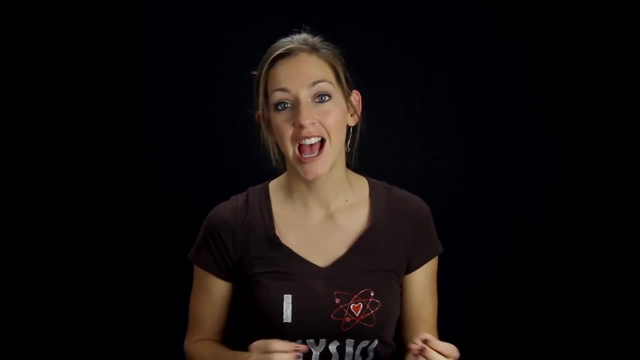 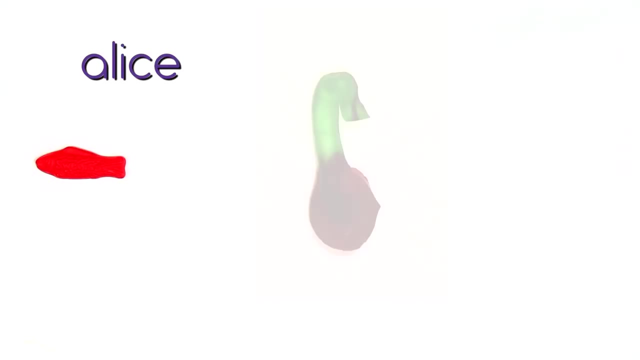 you use quantum mechanics to make one randomly and send it to your recipient. Here's how the random key is made: Alice, the message sender, sends photons that are polarized or vibrating in four different directions: Horizontal, vertical, diagonal, left or right. 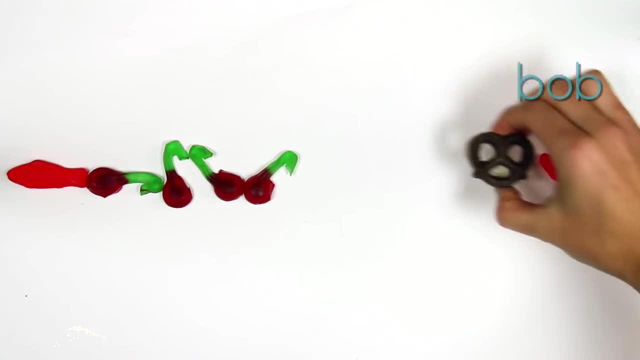 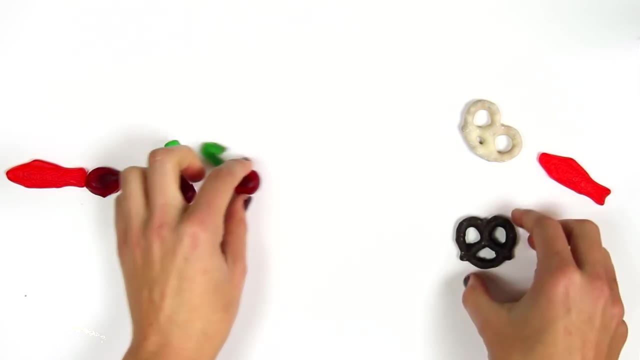 Bob. the recipient measures which direction they're polarized. Note- by using two differently polarized detectors for each photon, one at a time, back and forth, guessing which detector to use. randomly, the detectors translate the photons into bits, like a horse's tail. 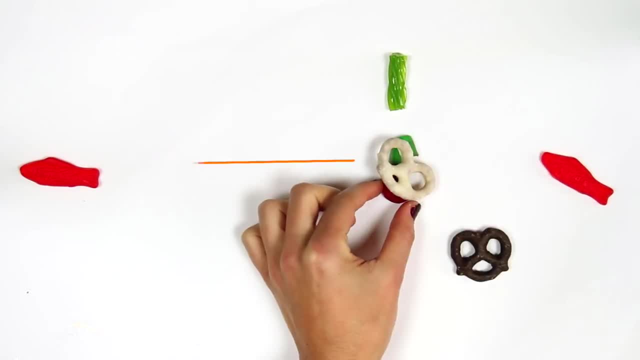 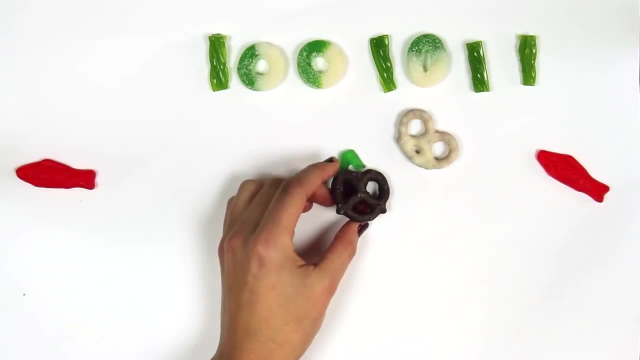 A horizontal measurement could register as a one and a vertical as a zero on this detector And eventually Bob will get the multiplication key from this set of bits. So now Bob has a measurement of one zero, zero one, et cetera. 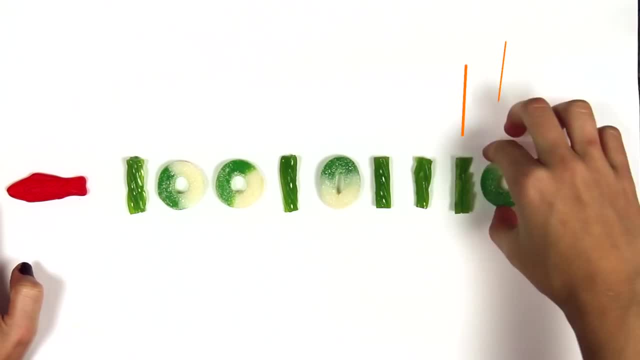 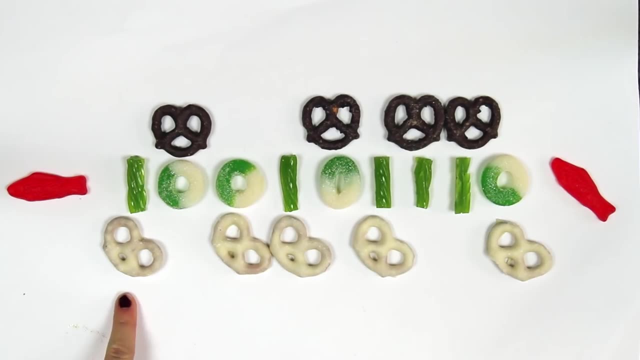 for each photon, keeping in mind that he measured them on two different detectors randomly. Now he compares with Alice and for each photon he'll tell her which detector he used and she'll tell him: wrong right, wrong right. 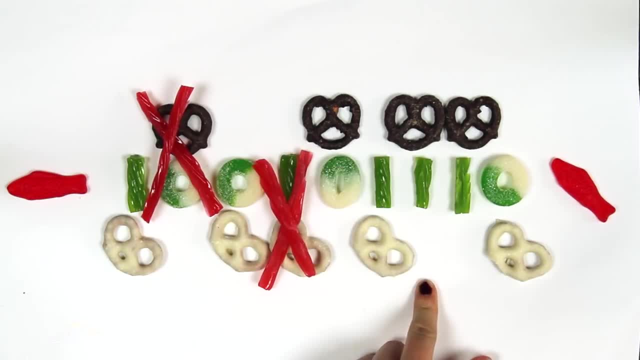 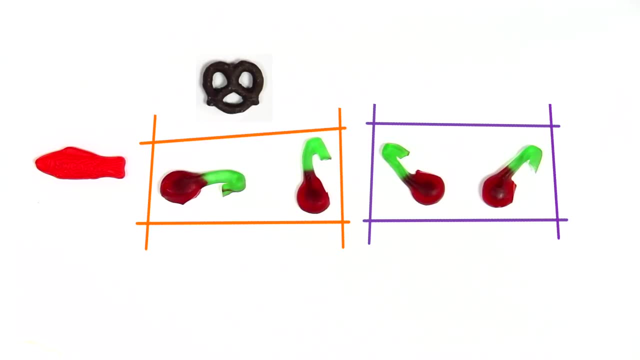 based on which filter she used to send the photons. Because, see, Alice sent either vertical-horizontal photons or diagonal photons And if Bob uses a diagonal detector on a horizontal or vertical photon, according to quantum mechanics, he will have a 50% chance of measuring a zero and 50% chance of a one. 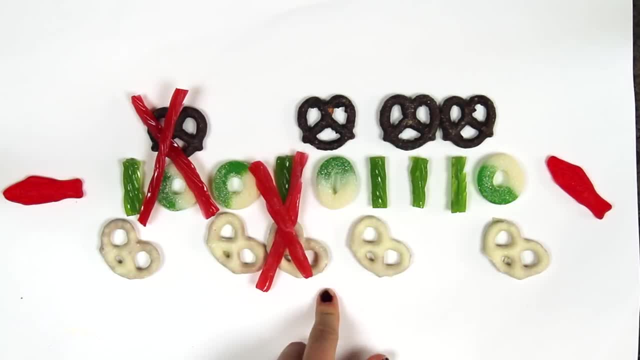 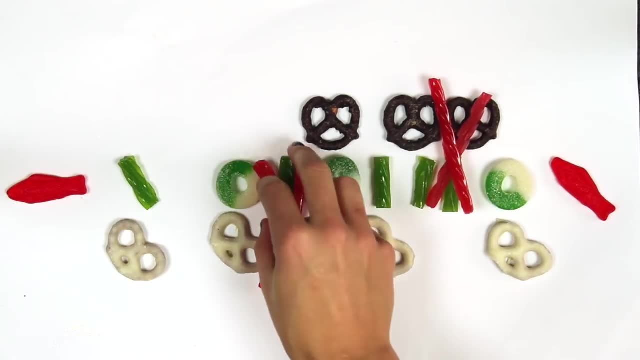 That's why Bob's detectors need to match Alice's filters After they go through this public check of the order the detectors were used. they throw out each result from when Bob guessed incorrectly and now they have a sequence of identically polarized and measured photons. 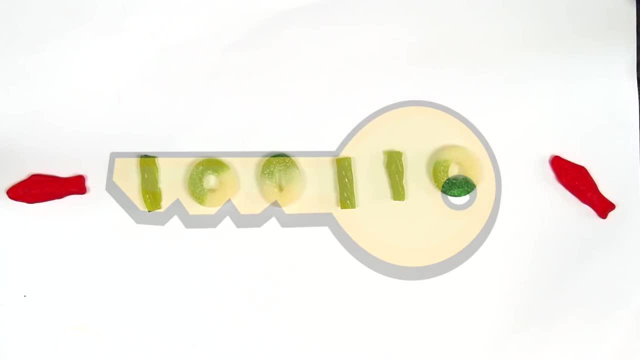 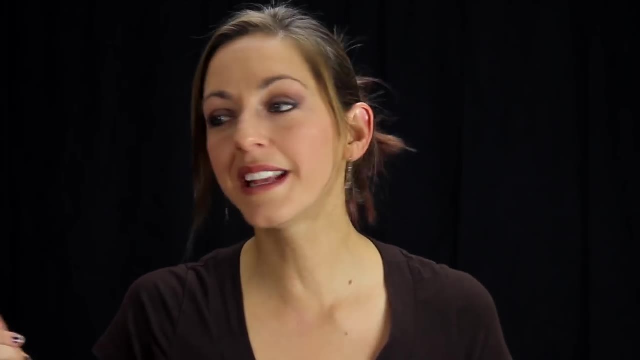 That sequence is the key. Alice can now send the actual encrypted message through a traditional channel and use the quantum key to decrypt it, And mathematicians have proven that if you make a truly random numerical key, you can theoretically make a code called a one-time pad that is unbreakable. 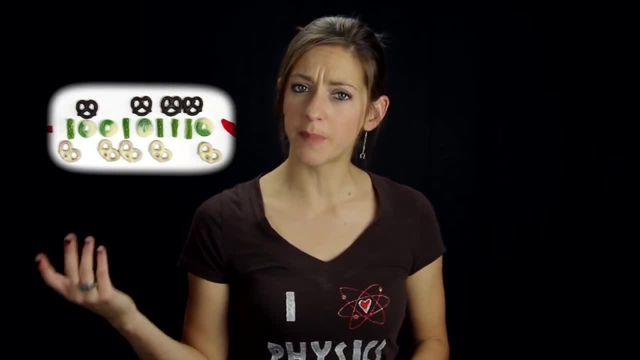 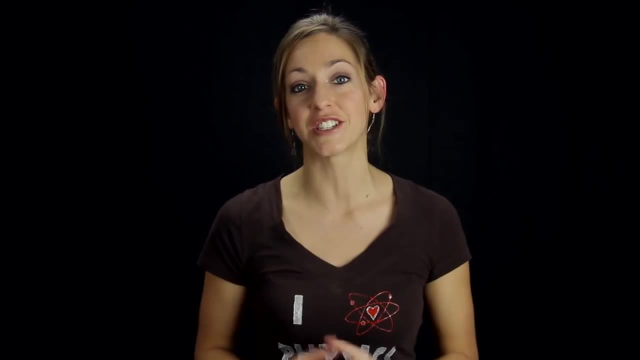 So why can the order of polarized detectors used by Bob be public? Well, it's not the ones and zeros that he obtains that are being shared. It's just the order of the ones and zeros that are being shared. It's the order of detectors. 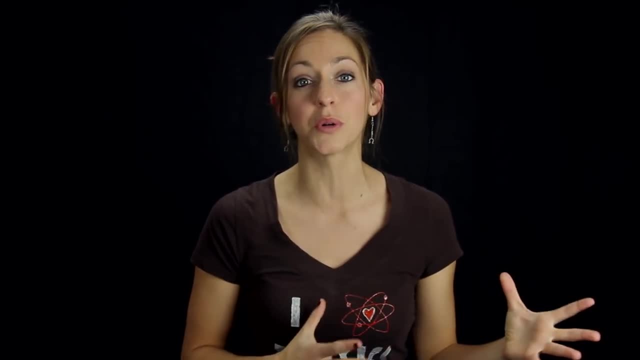 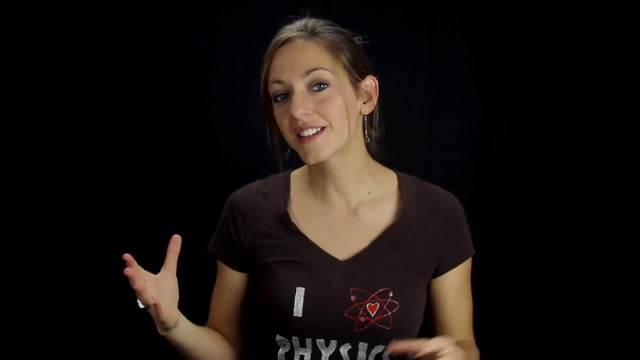 You would still need to send the polarized photons in through those detectors in the correct order to figure out the key, But those photons were polarized randomly, so the eavesdropper is out of luck. And things on this scale, a thousandth of the width of a human hair. get weird, as they say, because of quantum mechanics. If an eavesdropper hacks into the system and tries to copy some of the photons using the wrong order of detectors, they'll change the key. Bob and Alice will know, because they can check for errors. 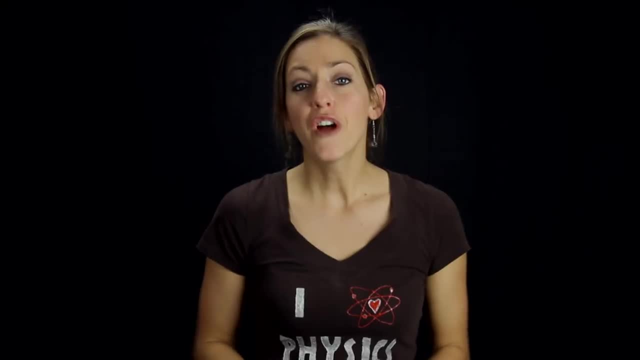 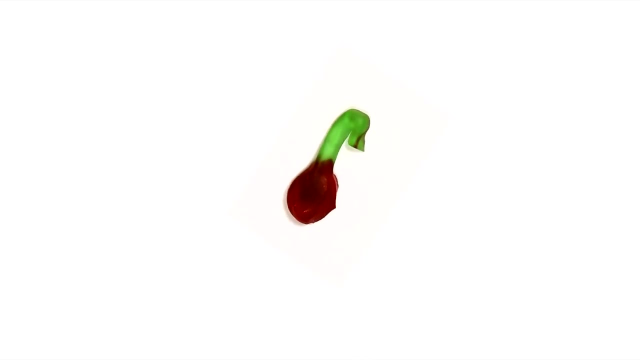 in a subset of the bits in the key and they can try again. Of course, getting quantum cryptography to work in the real world is not so easy. Small disturbances can change photon polarization And when creating photons, if you get them off by even just a degree. 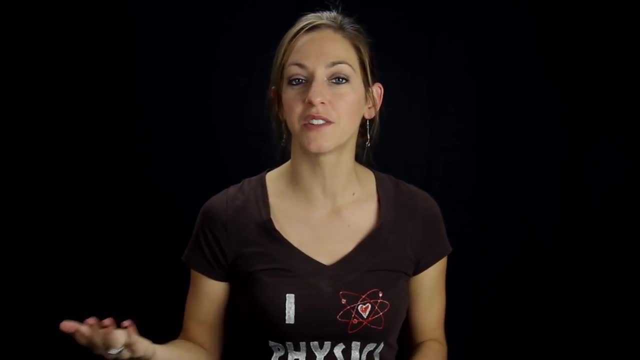 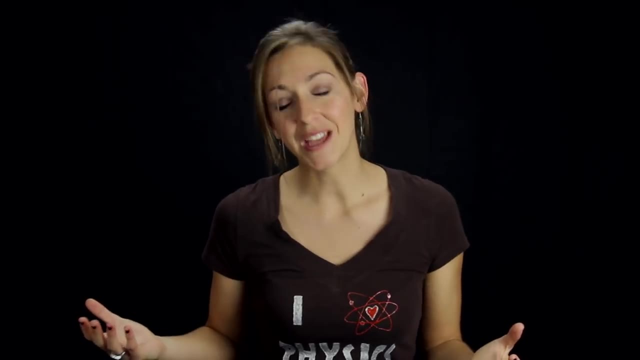 those errors will add up. Physicists have only been able to send quantum keys over 200 kilometers. You can even sabotage quantum detectors by shining a bright light on them, And even if quantum encryption does become commercially viable, much of the Internet's infrastructure.